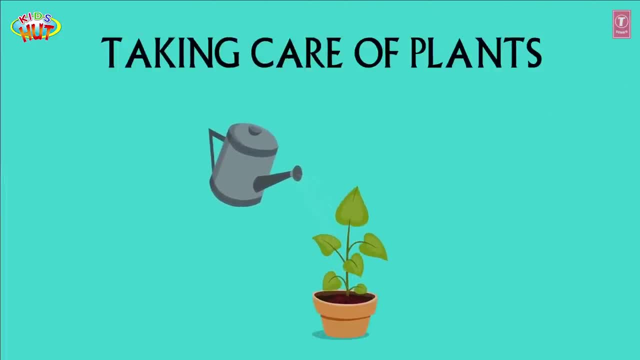 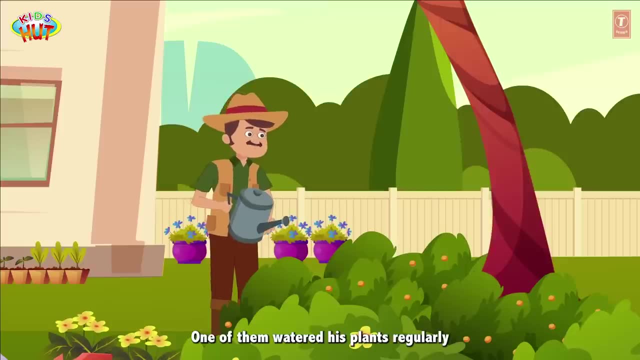 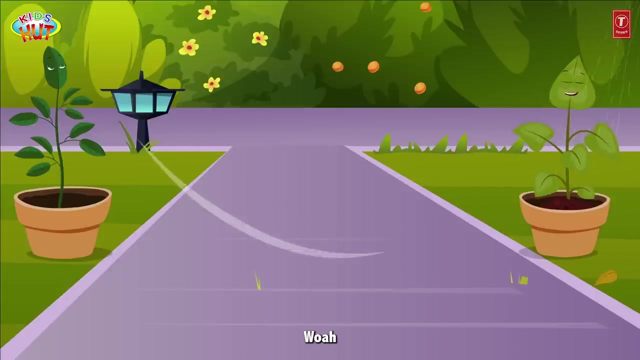 Taking care of plants. Once upon a time there lived two neighbours who were very fond of plants. One of them watered his plants regularly and the other one didn't. Whoa, The breeze is so swift. I am loving it. Oh God no. 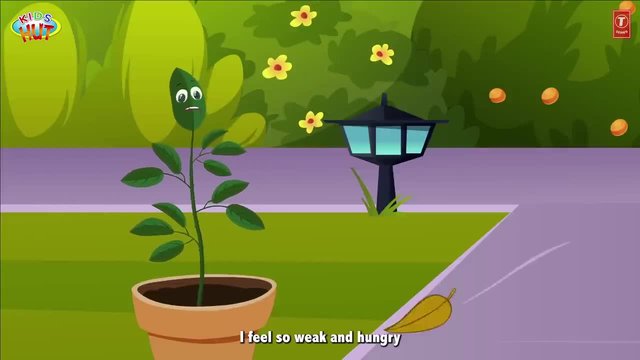 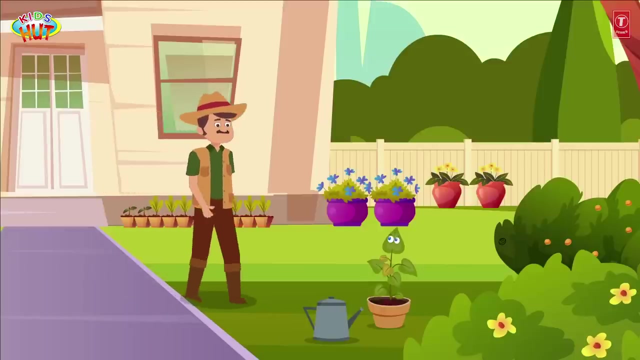 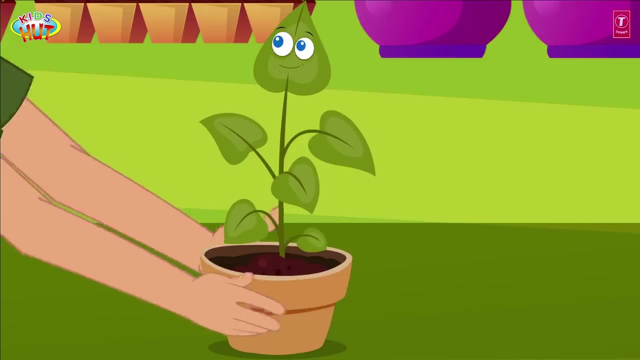 I am afraid I might break my stems. I feel so weak and hungry. Why are you hungry? Doesn't your owner feed you? I am afraid not. I feel I might break down very soon. Wee, I love the warm sun. 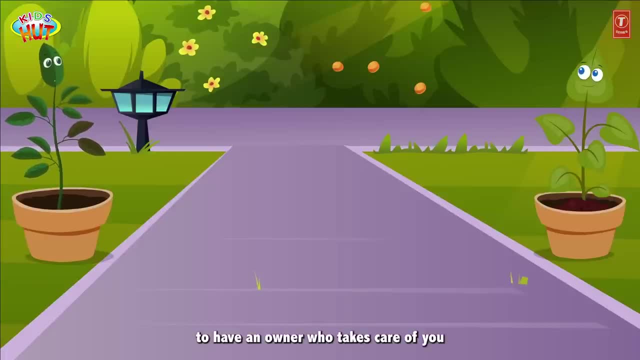 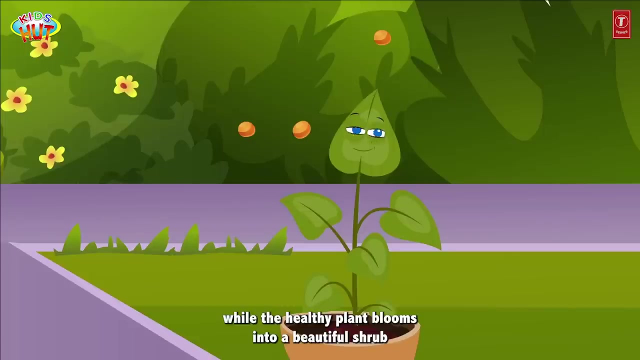 You are so lucky to have an owner who takes care of you. Look at me. I fear I might not live for long. My owner doesn't take care of me at all. The unhealthy plant withers day by day while the healthy plant blooms into a beautiful shrub. 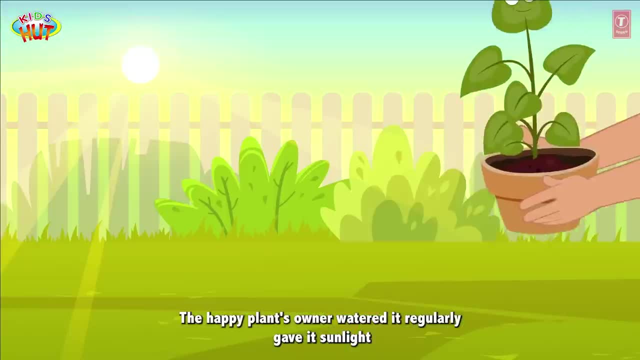 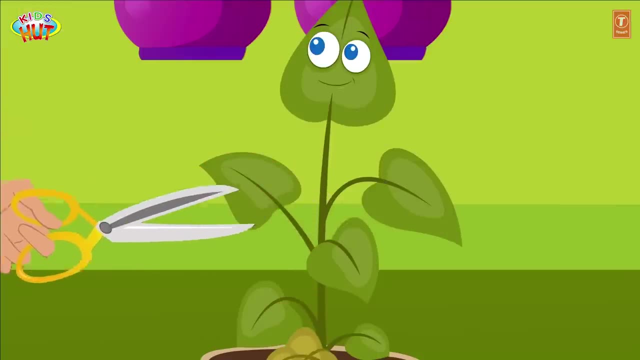 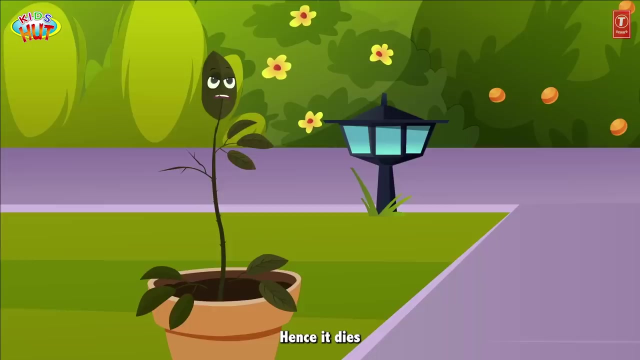 The happy plant's owner watered it regularly, gave it sunlight and cleaned it too. On the other hand, the withering plant's owner neglects it and forgets to feed it, Hence it dies. Tia, this is so sad. 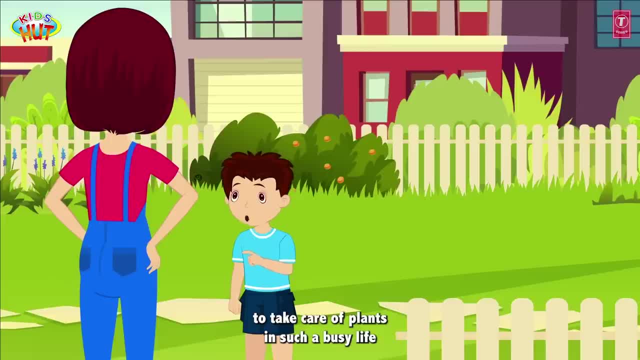 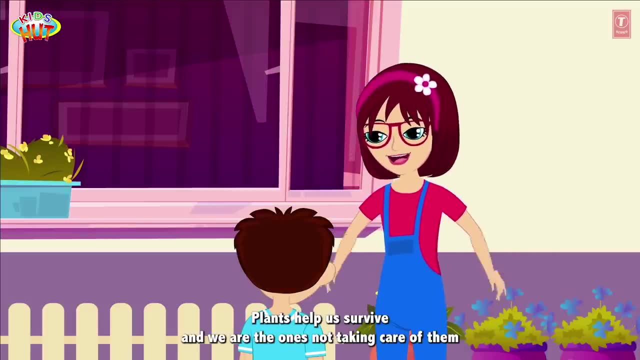 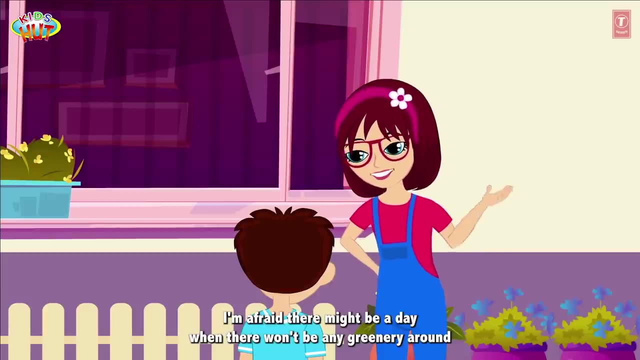 There must be so many people who forget to take care of plants in such a busy life. You are right. Tofu Plants help us survive and we are the ones not taking care of them. I am afraid there might be a day when there won't be any greenery around. 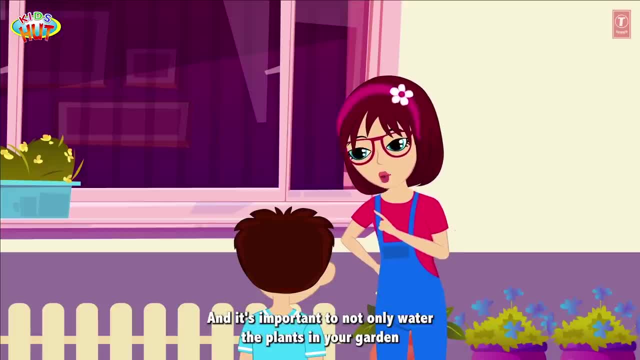 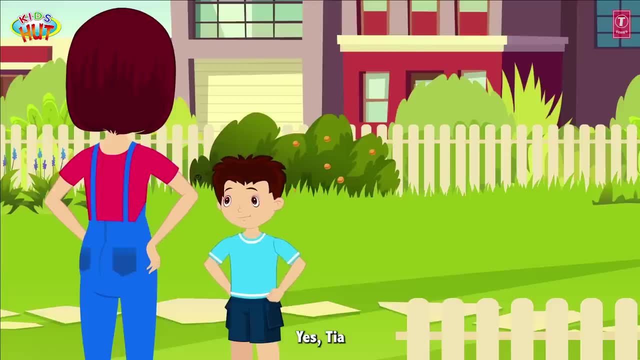 And it's important to not only water the plants in your garden, but in public places too, where you might feel the plants are neglected. Yes, Tia, I will take care of it. From tomorrow, I will water the plants every single day. 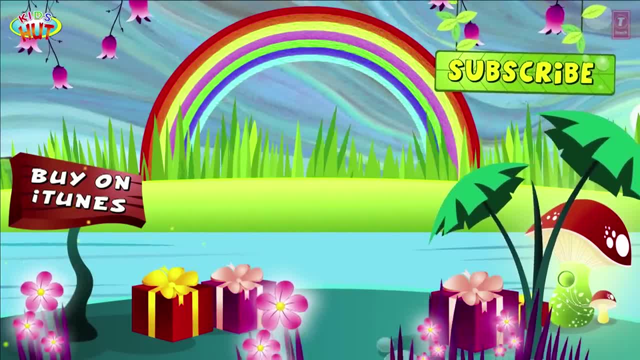 Thank you, Thank you, Thank you very much, Thank you, Thank you.